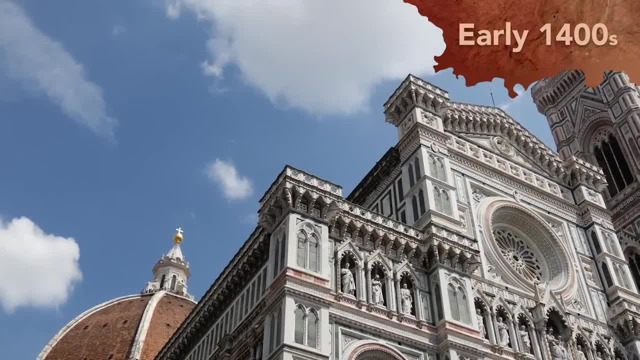 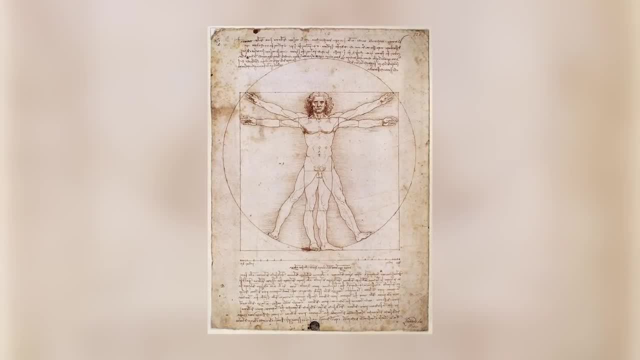 around the first half of the 15th century in the early Renaissance, when the cultural movement of humanism became the rage. Humanism in the Renaissance focused on, as its title suggests, humans, their values, agency and individual worth. 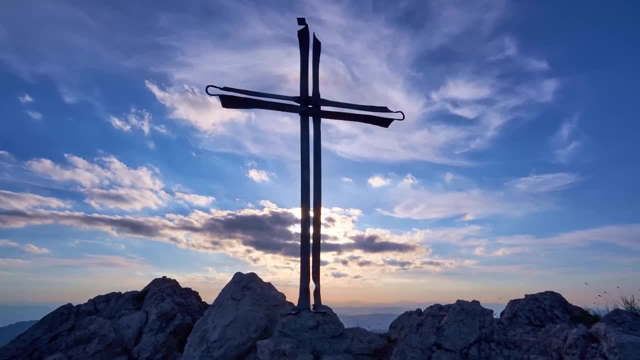 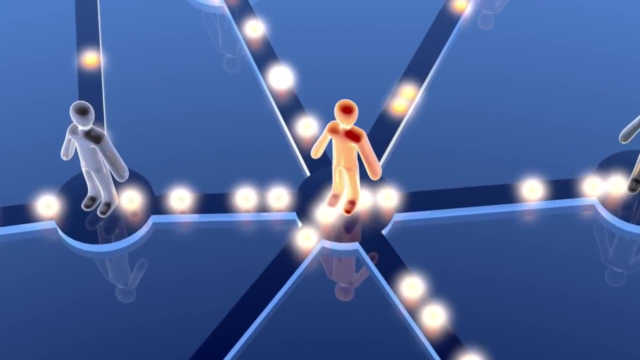 Humanism started as a movement to renew Christianity from the complicated theology of the medieval period. It included a belief in the individual's ability to achieve excellence, especially through the study of art and literature of classical, Greek and Greek culture. As a result, literature, art and philosophy 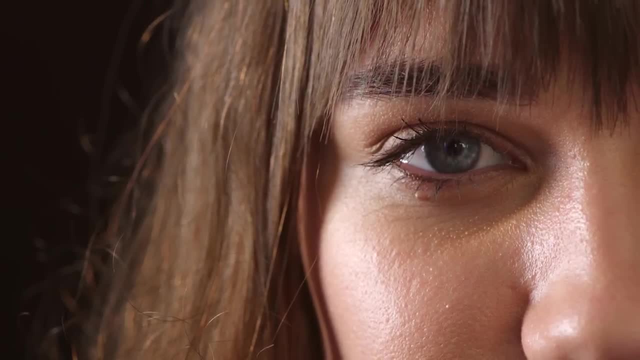 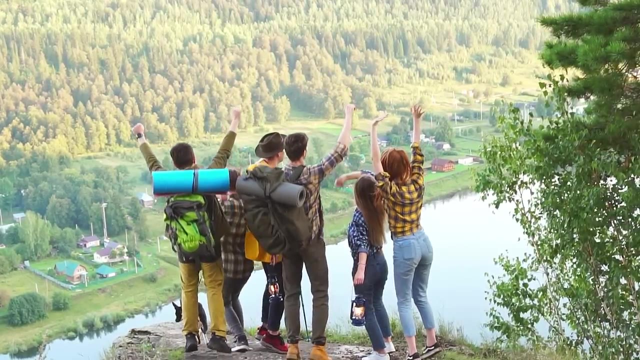 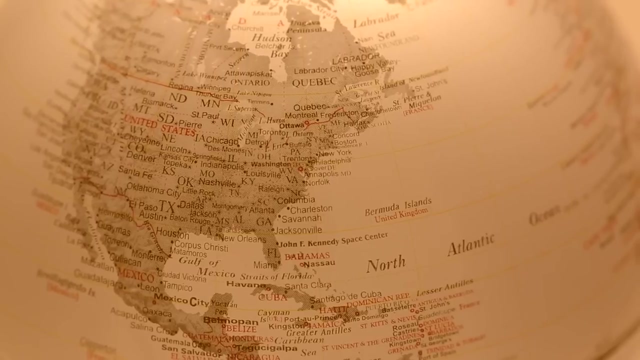 shifted focus from cosmic concerns to the human perspective and individual expression and achievement. In other words, people began to believe human life and accomplishment had inherent value. That's a nice concept. Oh my Sex Depending on when and where you lived in history. 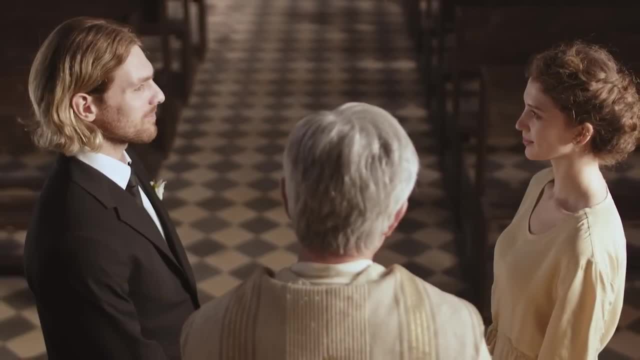 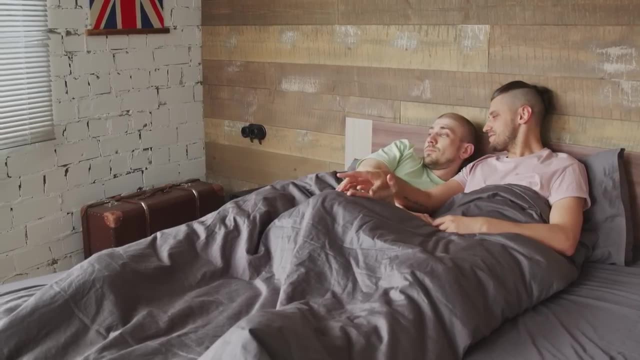 sex could be viewed in many different ways, ranging from a sacred, transcendent union to a dirty necessity, to just a little bit more. Sex was often considered, eh, just another chore, Because at that time the common understanding of anatomy led them to conclude women could not get pleasure from sex. 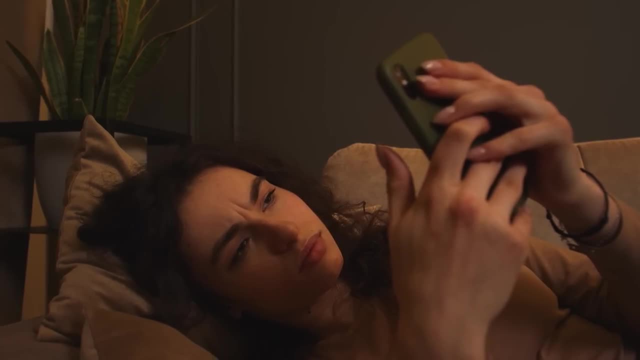 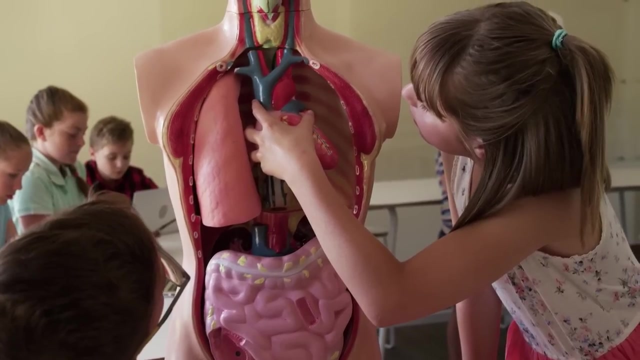 I wonder if those anatomists knew any actual women. But as the Renaissance progressed, views changed, both by advances in anatomy and well practical experience, And sex was seen as an activity men and women could enjoy. This led to more sex during the Renaissance. 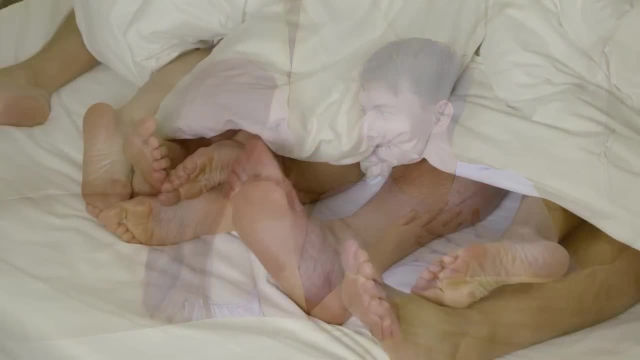 with those alive at the time of the Renaissance being the most popular. Sex was also seen as an activity that men and women could enjoy. Sex was seen as an activity that men and women could enjoy. This led to more sex during the Renaissance. This led to more sex during the Renaissance. 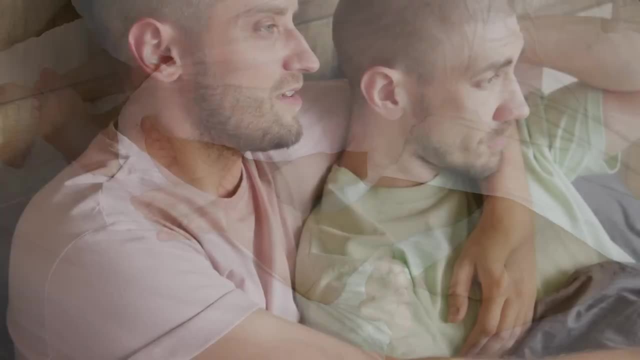 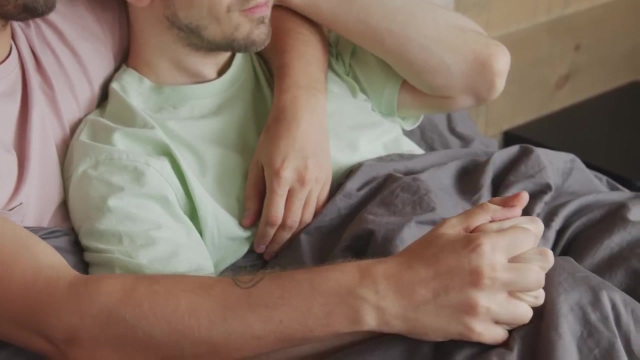 And the taboo of homosexuality, more common in ancient Greece And the taboo of homosexuality, more common in ancient Greece and Rome, made a minor comeback, partly due to the emergence of the hedonists, known as libertines, who eschewed any restraint in their pursuit. 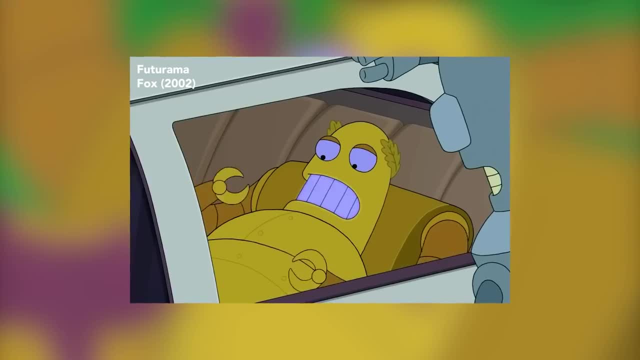 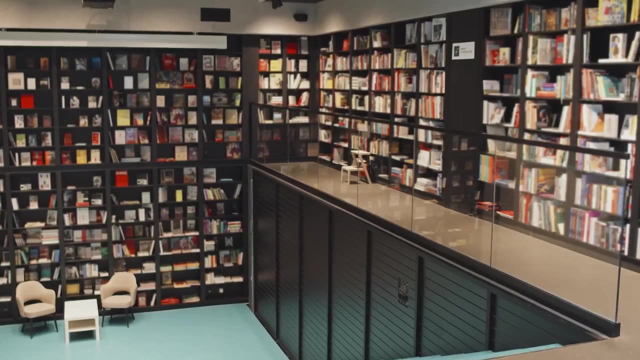 of earthly pleasures. Maybe that's where they got the idea for a hedonism bot from Futurama. Do you like to read? And we're not just talking about books or newspapers, We also mean road signs or menus or pretty much anything that has writing on it. 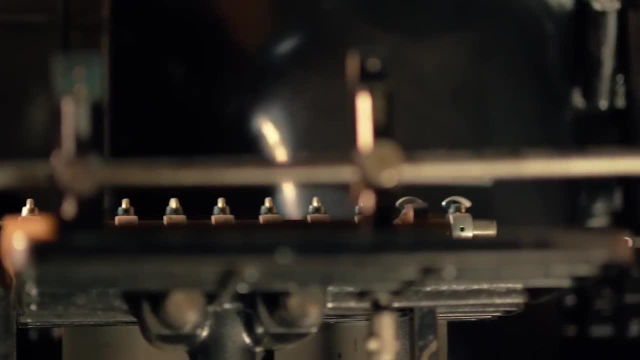 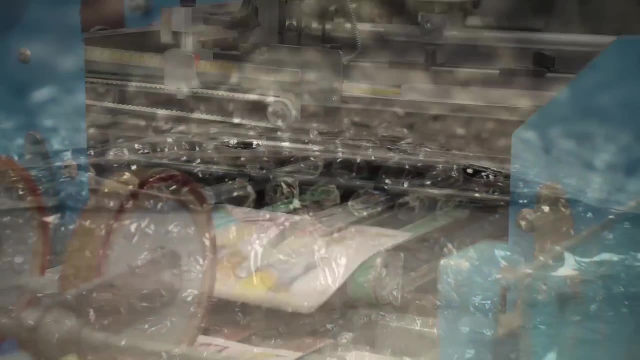 well, you can thank your lucky stars and asterisks for the printing press, which helped spread the written word. It's one of the most important inventions in the history of mankind, maybe more important than bubble wrap, And we owe it to a man named Gutenberg Johannes. 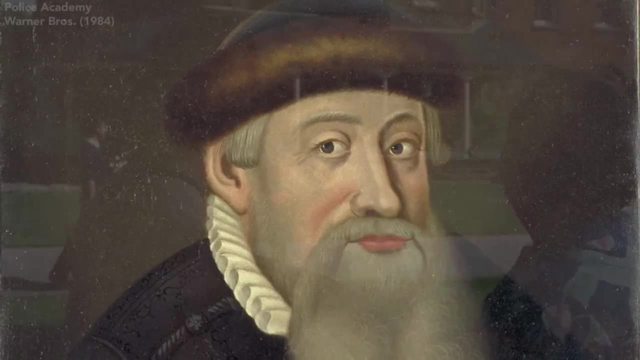 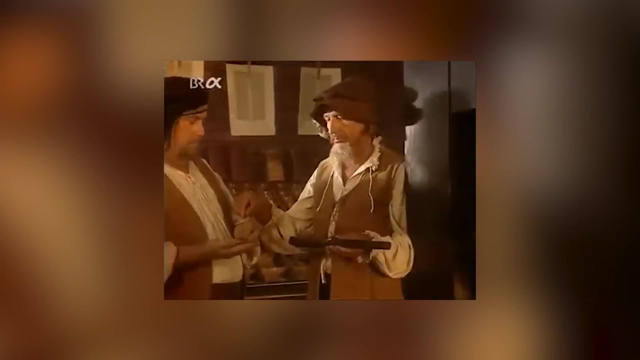 Gainsflash-Zurladen zum Gutenberg. that is Not the guy from the Police Academy movies, although we do owe that Gutenberg an equally immeasurable debt. Building on the work of previous inventors, Gutenberg invented his movable type press around the year 1440.. 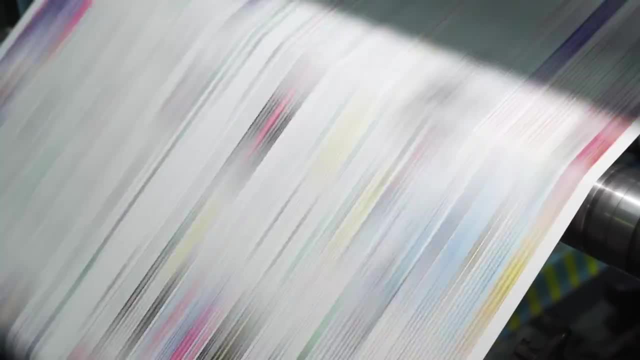 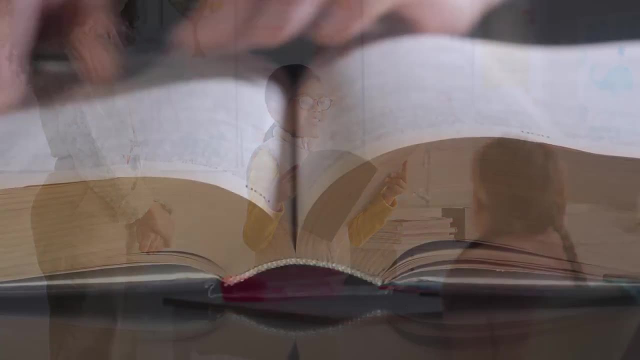 The printing revolution followed, enabling the mass publication of well basically everything. This made books available to the masses, led to increased illiteracy and paved the way for evolution in education by allowing for the production of textbooks. As for Gutenberg, his achievements: 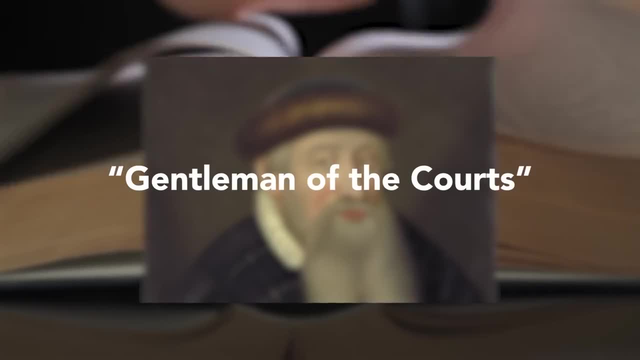 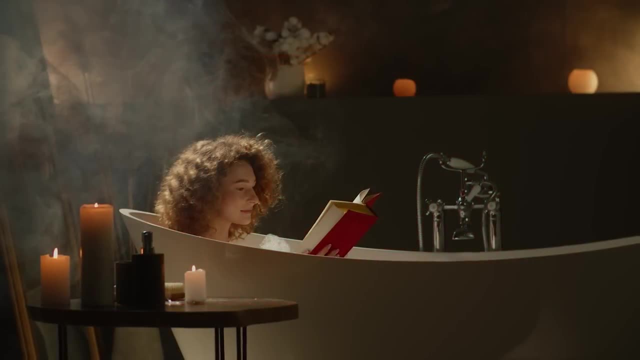 were recognized with the title Gentlemen of the Courts. Among other things, the honor included 2,000 liters of tax-free wine. We can only imagine he celebrated by sipping that wine while reading a steamy romance novel In the bath. 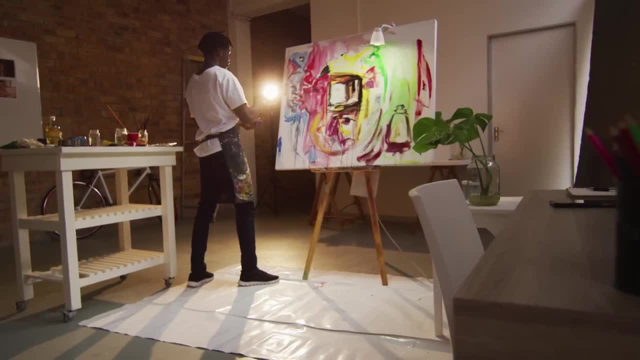 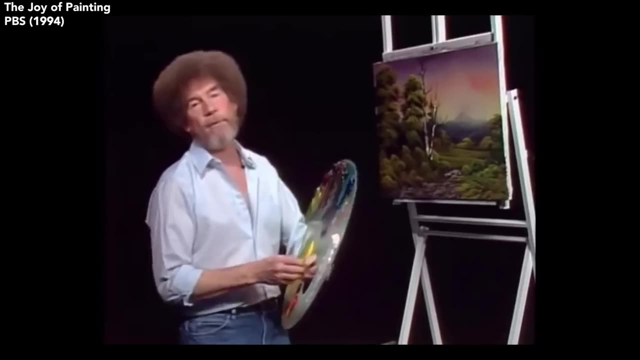 If someone asks you to picture an artist, there's a good chance. you're picturing someone like Bob Ross: Brush in hand, palette on arm, a working canvas and hair like Art Garfunkel. Well, you're picturing a Renaissance artist. 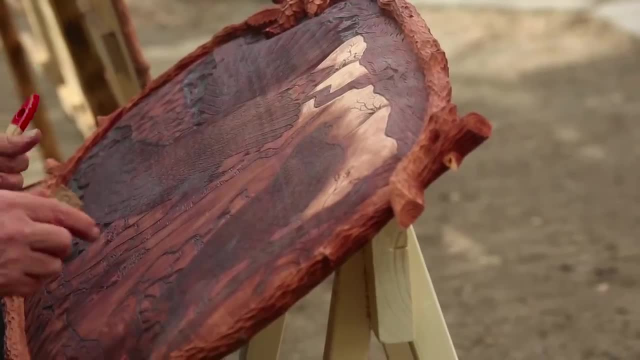 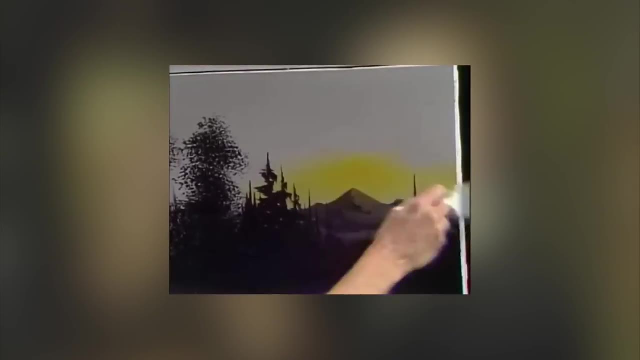 But prior to the Renaissance in Europe, painting was typically done on wood panels. Renaissance artists introduced the idea of painting on canvas And that's why you've never seen Bob Ross paint a 2 by 4.. And prior to the Renaissance, painting often 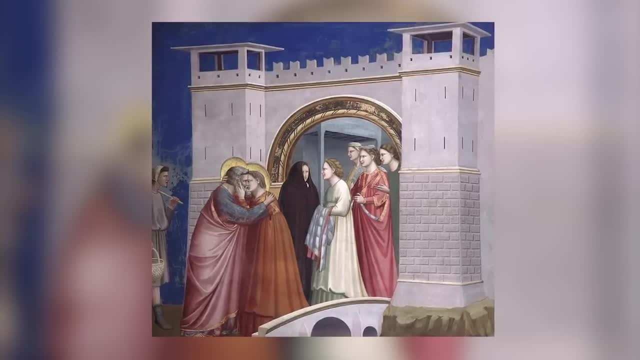 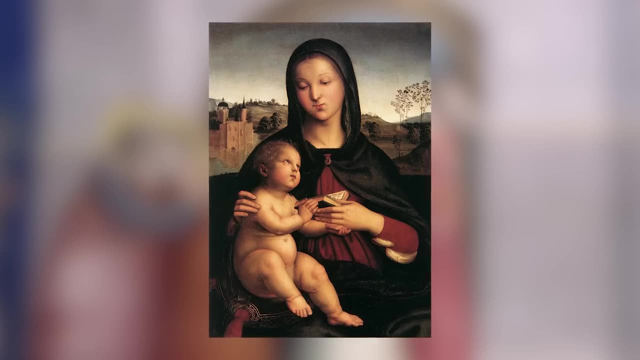 relied on symbolic language, where the relative size, placement and depictions of people and objects had more to do with their meaning rather than what they actually looked like. But advances during the 15th century changed art, And painting became more representative of what 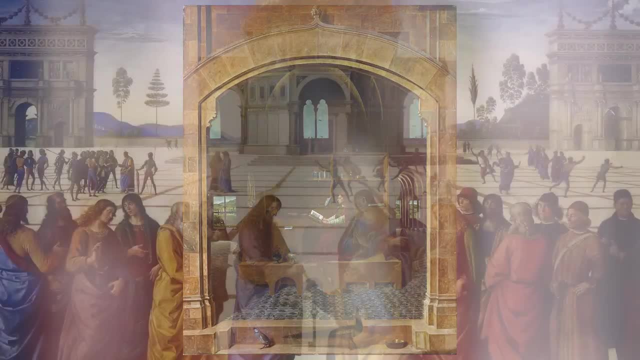 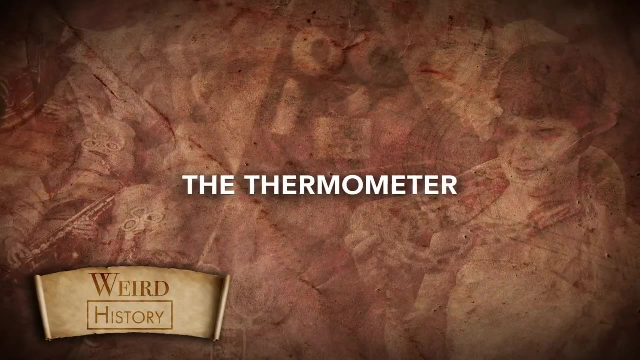 a human actually seeks exploiting advancements such as linear perspective, And that eventually leads us to happy little clouds. Thermometers are so ubiquitous that they're not only used in the art of painting, but they're also used in the art of painting Thermometers. 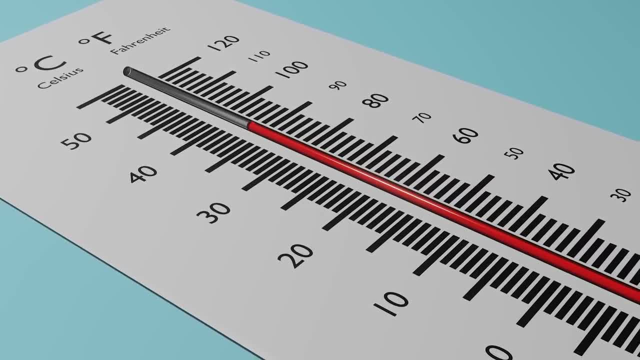 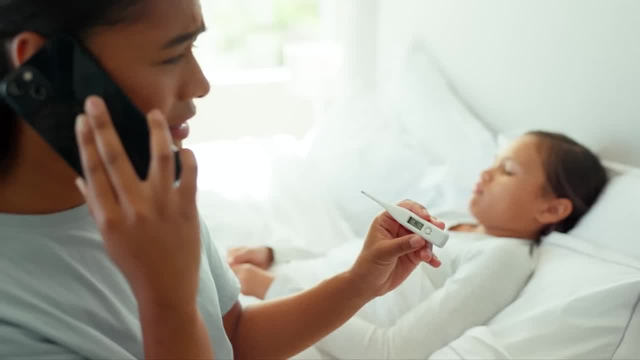 Ubiquitous in modern society. it's weird to think that those handy devices weren't readily available to ancient people, Although that did make it easier for ancient children to skip school by faking being sick. Luckily, the Renaissance came along with its good citizen. 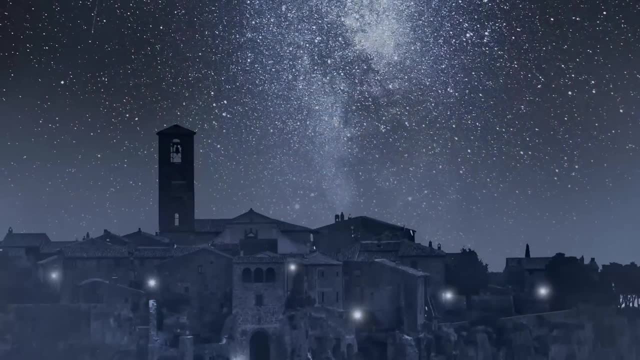 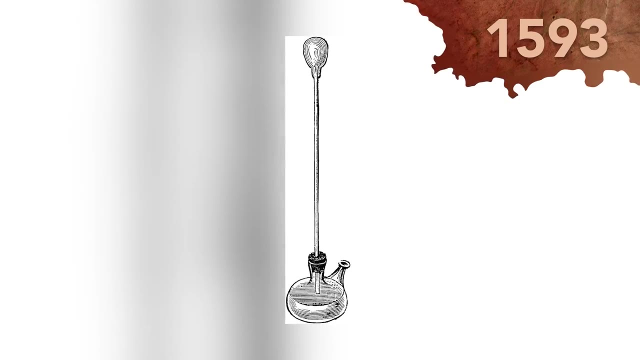 Galileo Galilei. He's mostly known for his contributions to astronomy and being forced to recant his contributions to astronomy, But in 1593, he also developed a device we would recognize as a rudimentary thermometer, which he called the thermoscope. 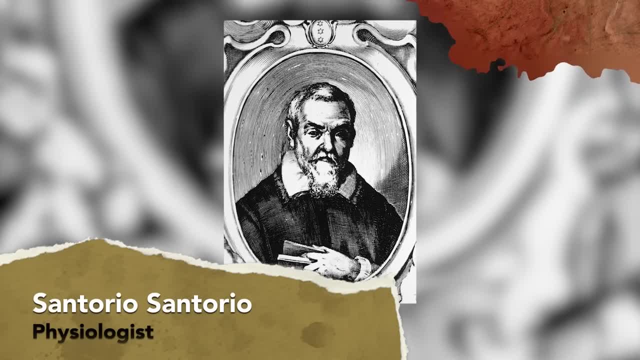 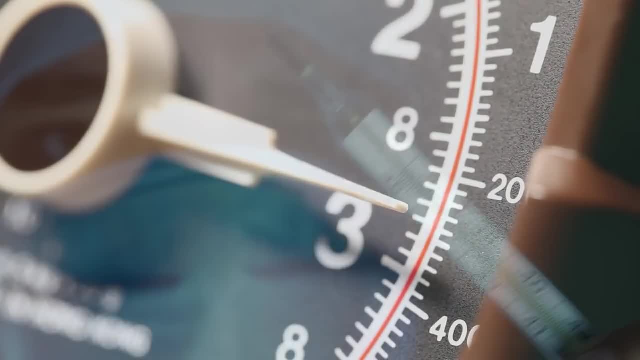 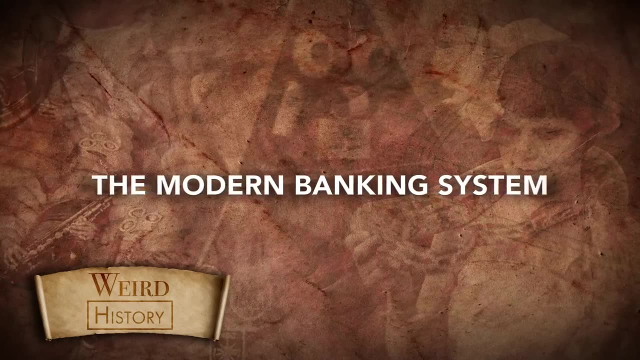 Ooh, so close. Galileo In 1612, Santorio Santorio, who perfected Galileo's same name twice style, added a scale to the thermoscope, transitioning it into what is now recognizable as a thermometer. Is there anything cooler than living? 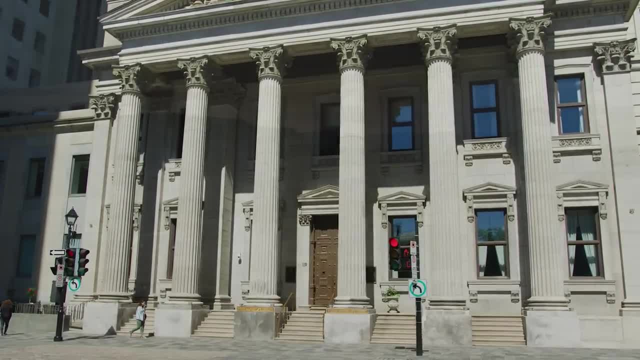 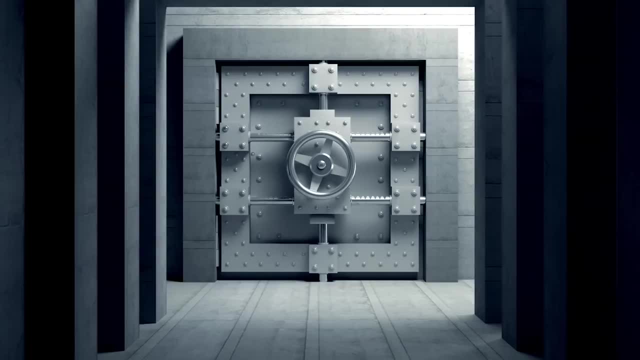 close to a branch of your bank? Oh yeah, there definitely is, But it's still pretty convenient that you don't have to drive all the way to your bank's national headquarters to deposit your paycheck. And one reason banks have branches is because of a famous Renaissance. 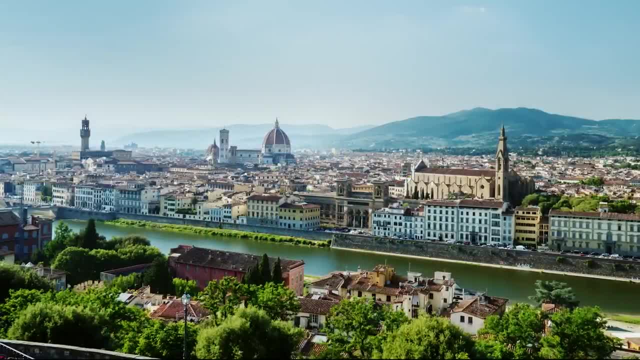 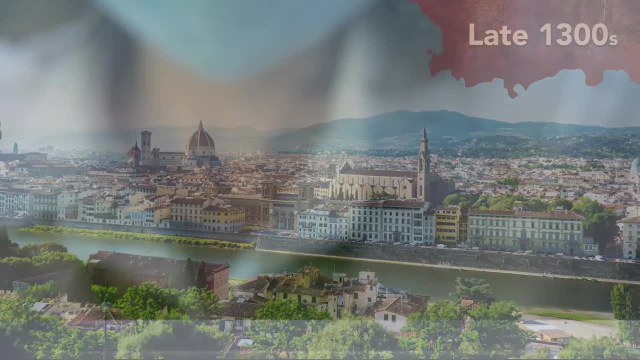 family, the House of Medici. The Medici were a powerful family from Florence, Italy, who rose to prominence at the end of the 14th century. They were all about increasing their wealth, And one way the wealthy get wealthier is to give loans to people and attract their finances. 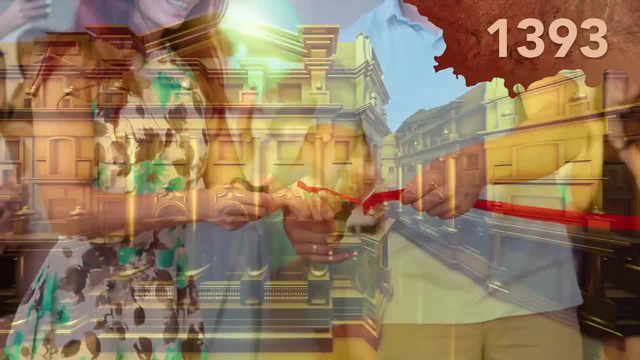 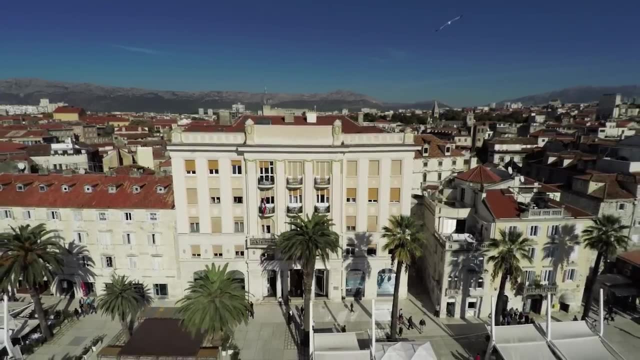 The Medicis opened their first bank in 1393 and began expanding soon after, opening branches in different cities. The rest of the world knew a good thing when they saw it, And today that's pretty much how everyone does it. Incidentally, the Medici were also major patrons of the arts. 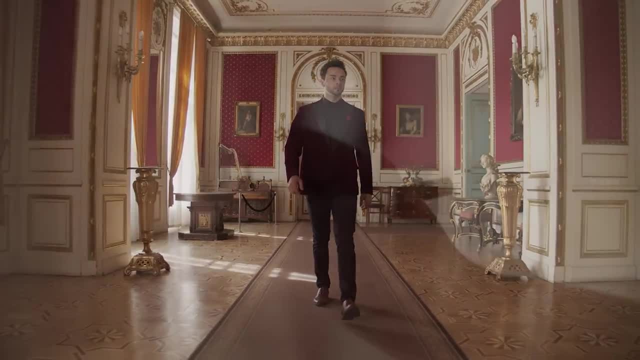 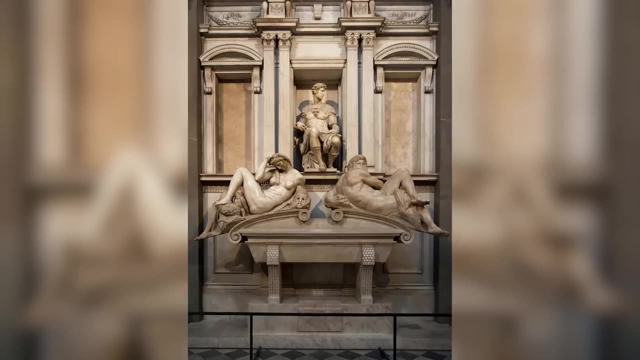 The gig you can really only get if you're super filthy rich. The family commissioned some of the most important works of art and architecture in history, including Botticelli's Birth of Venus, Michelangelo's Tomb of Lorenzo de' Medici and the Uffizi Gallery in Tuscany. 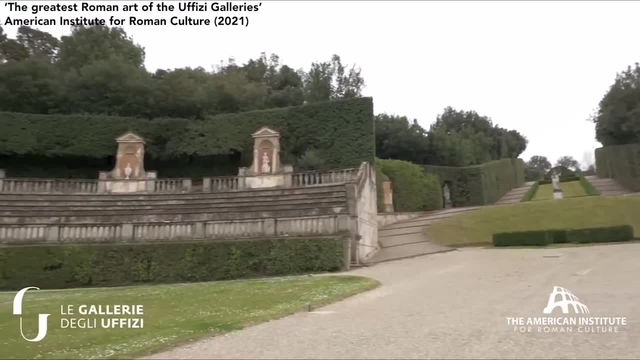 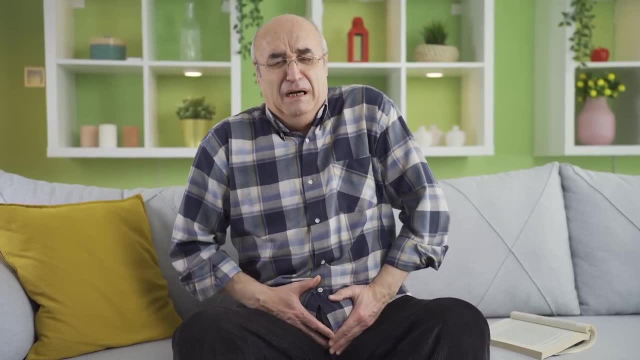 So thank them for that too, when you order your custom Birth of Venus checks. One of the best parts of modern life is that when you have to relieve yourself, you don't have to go find a hole in the ground or a bush you. 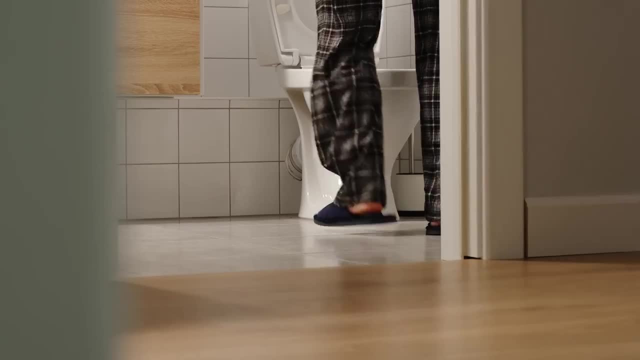 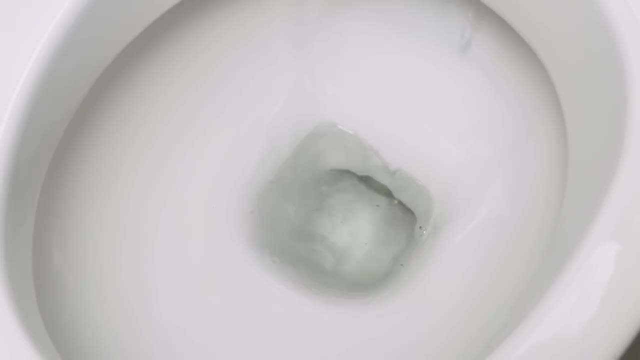 dislike, You can just go to the bathroom, do your business and then whisk the evidence away down a toilet, And this is all courtesy of the Renaissance. In particular, you could thank the failed poet, Sir John Harrington, the godson of Queen Elizabeth I. 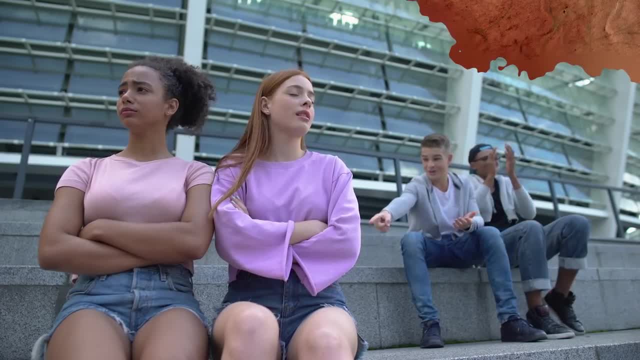 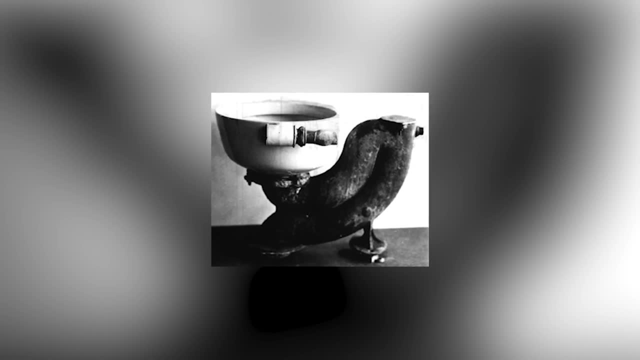 Harrington had been banished from court for telling too many dirty jokes, And it was in 1591, while he was in so-called exile at Kelston near Bath, that he invented a strange device that could flush waste away to another location. He first called it Ajax, And if you call it the John, Sir John Harrington is why The queen got over her distaste for dirty jokes and got one for herself. But strangely toilets didn't catch on until centuries later. No one even bothered patenting it for another 200 years. 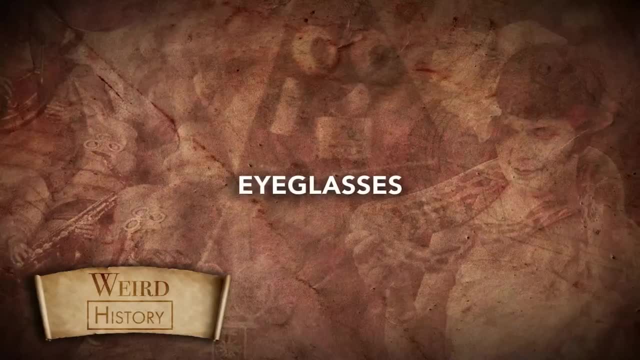 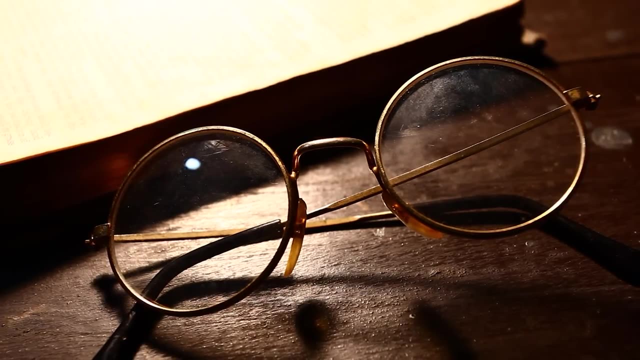 flushing away lots of potential dough. If you're watching this video through a pair of glasses or contact lenses, guess what You have the Renaissance to thank. Throughout the era, eyeglasses were changed, adapted and tested to be more effective. 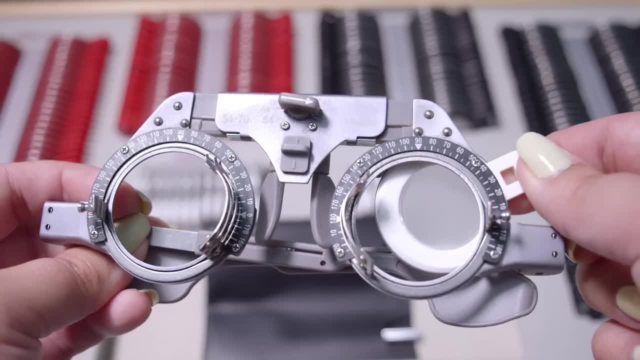 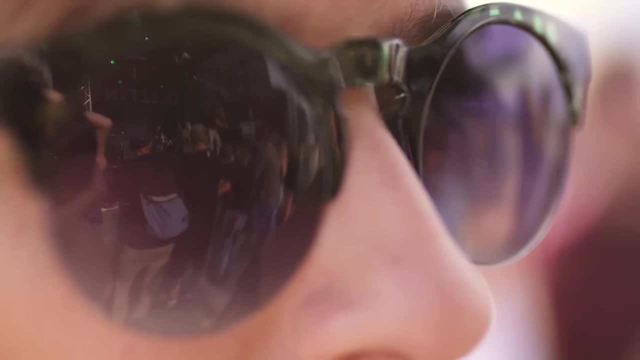 Not only was this a huge deal for people with eye problems, but it also tipped the fashion world on its head. Elton John was far from the first person to discover what a pair of glasses can do for your appearance. Innovators in the field also messed around. 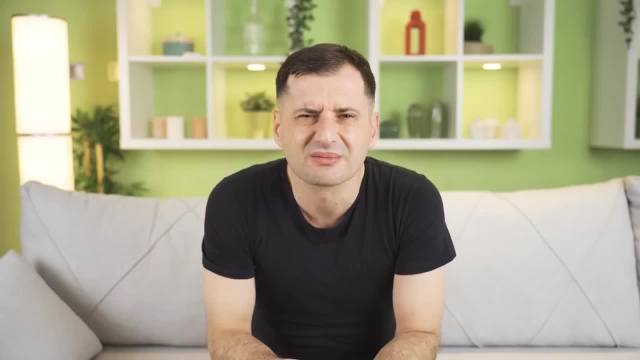 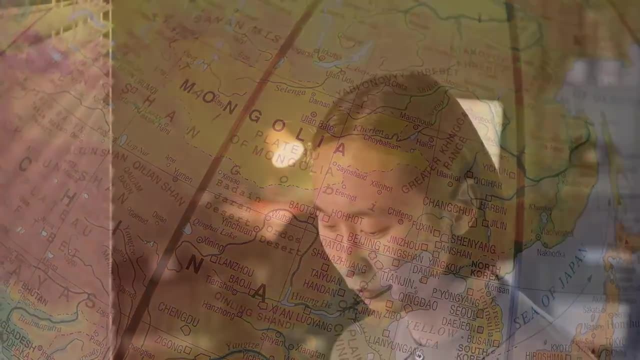 with tinting lenses in an effort to cure or at least alleviate various visual problems and impairments. Some of these developments were due to increased contact with the Far East, where the Chinese were responsible for a number of ocular innovations, including the use of cords or loops. 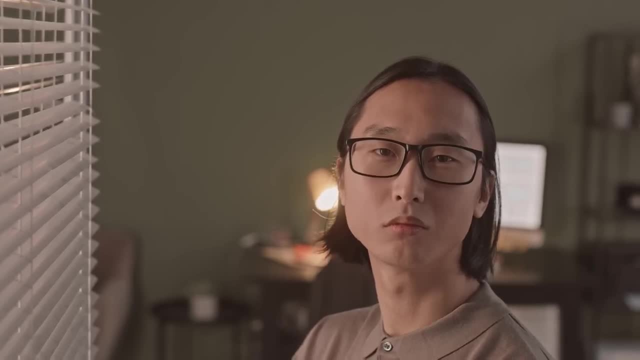 to fasten the glasses to the ears and keep them on the floor, And some of these innovations were also due to the fact that the eye glasses were used as a way to protect the eyes from the face, So, in many ways, modern eyeglasses. 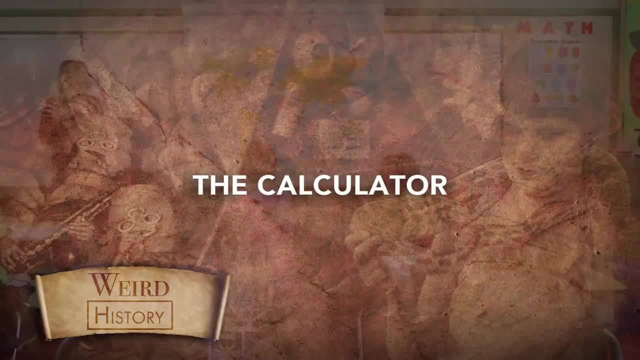 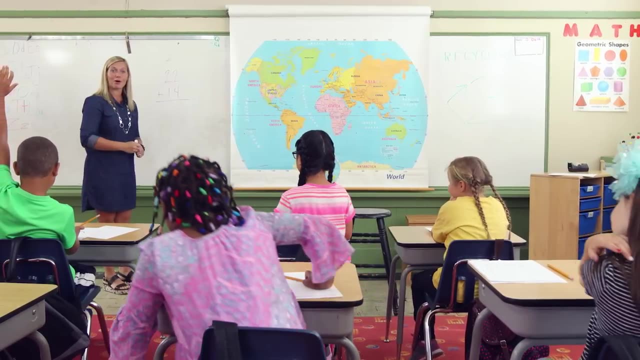 are kind of the result of a globalized effort. Go team Earth. Once upon a time, teachers insisted that students need to do math in their heads, under the theory that they wouldn't always have a calculator available to them. Of course, that was before everyone, really. 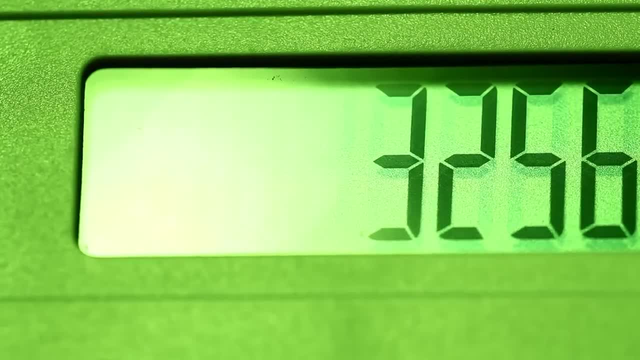 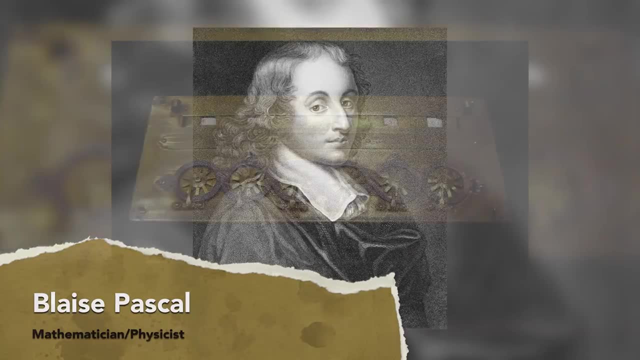 did start carrying calculators with them everywhere they went, Calculators that can also be used as phones. How handy. Take a fellow named Blaise Pascal. In the mid 1600s, he was the first to develop and manufacture a mechanical calculator. because he 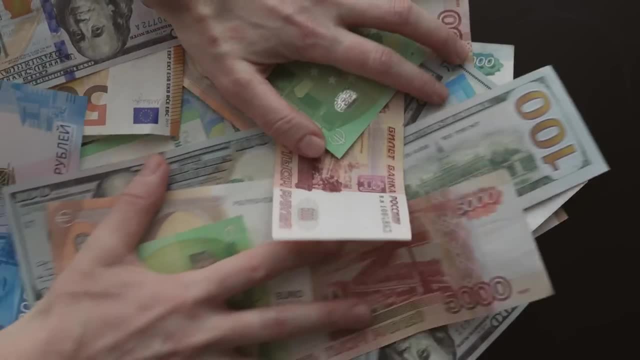 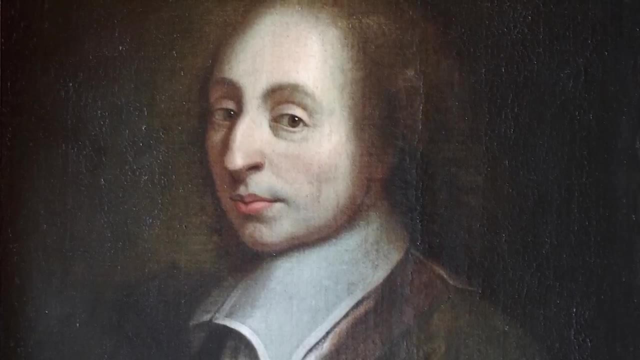 wanted to help his dad with some tricky math. Unfortunately his dad was a tax collector, so he's a little hard to root for. But Pascal himself was a mathematical genius, physicist and philosopher, So just root for him. He developed that mechanical calculator when he was just 18. 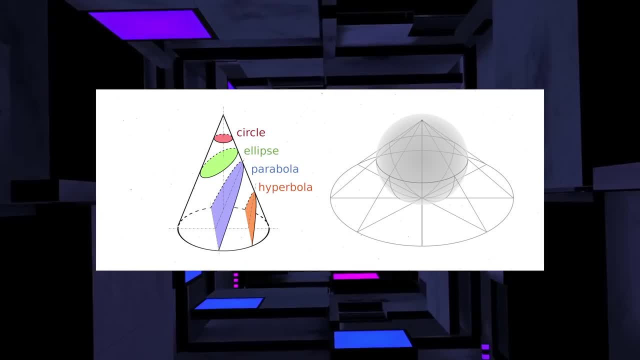 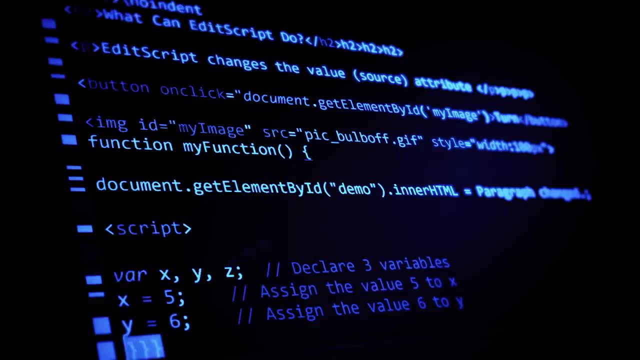 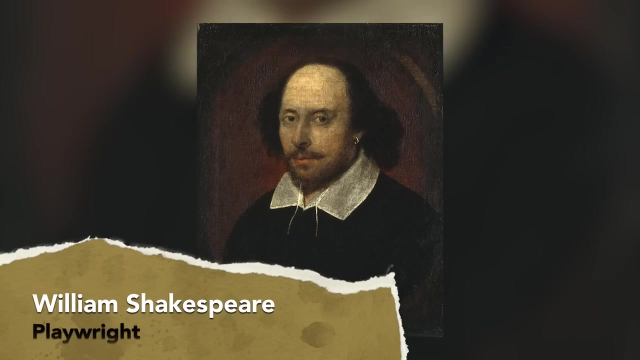 and then did important work on conic sections and projective geometry. Today his name is widely known thanks to being attached to a computer programming language. We're guessing he would approve. Also known as the Bard of Avon, William Shakespeare was quite possibly the most influential writer. 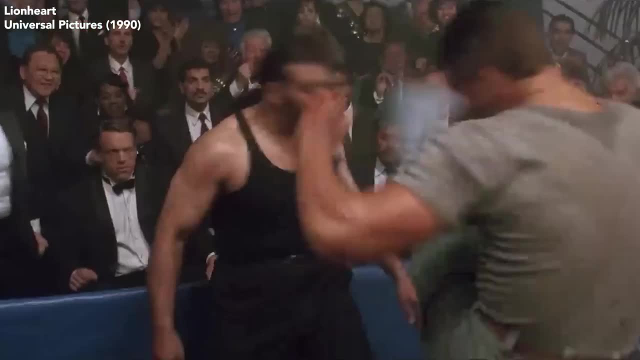 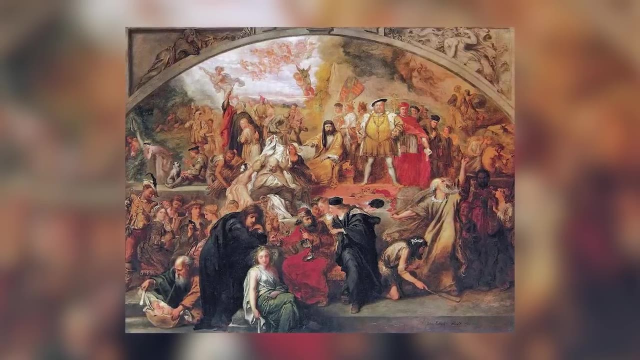 to ever wield the English language, And he wielded it like Jean-Claude Van Damme and a good pair of boots. In addition to being classics in their own right, his works are the foundation of numerous contemporary dramas. House of Cards is just Macbeth.